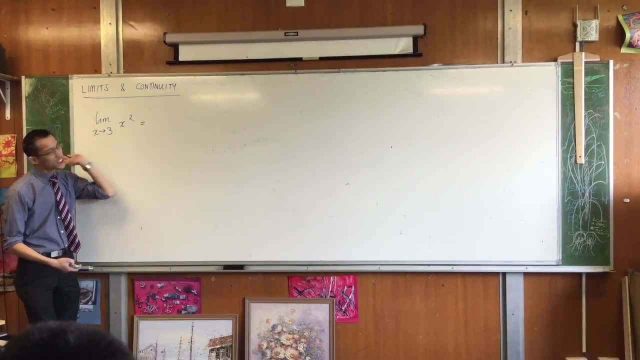 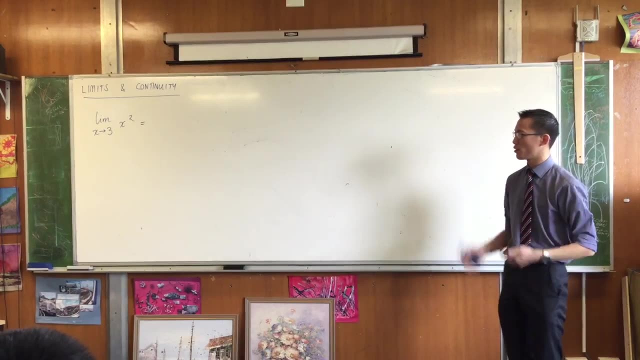 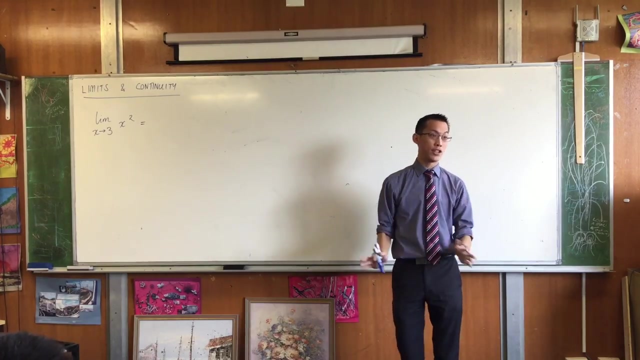 Limiting continuity is the heading. These are ideas that I have sown the seed about and talked about informally over the last week or so, But now it's time to do this in what mathematicians call a rigorous way. We're going to get watertight, detailed, formal definitions for all of these things. 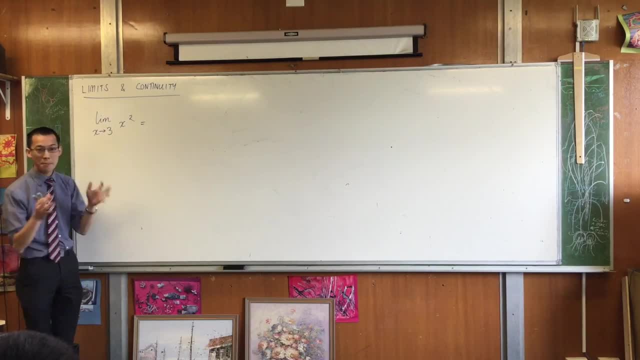 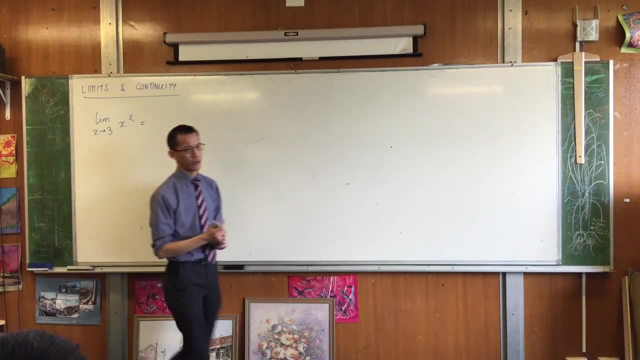 Both of these hang together, even though they are quite big ideas, So it makes sense to introduce them simultaneously. This thing here, really kind of new notation. I'm going to read it out for you. I'm going to tell you how I read this. 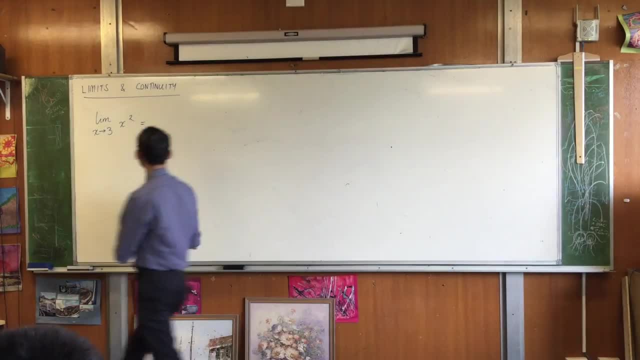 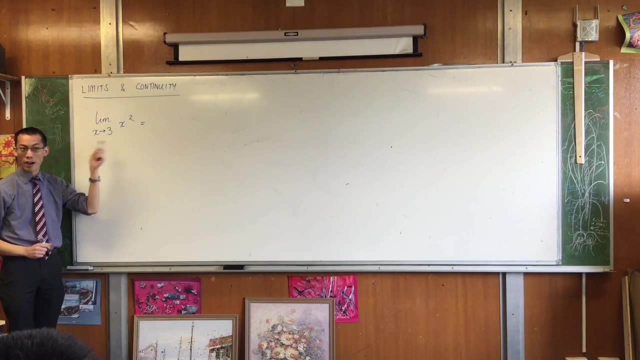 And then you're going to tell me what the number is. So the way I would read this is- and I'd love you to write this underneath so that when you refer back to this in like three or four or five weeks, when it's been a while since you've touched this- 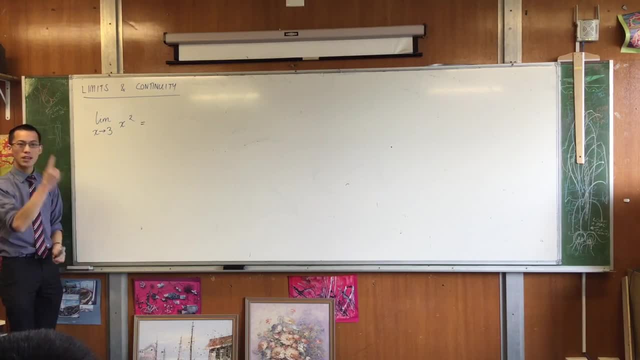 you'll be like: oh yeah, this is what that weird notation was talking about. The way I would read: this is the limit. that's what the lim is. lim is short for the limit as x approaches, in this case 3,. 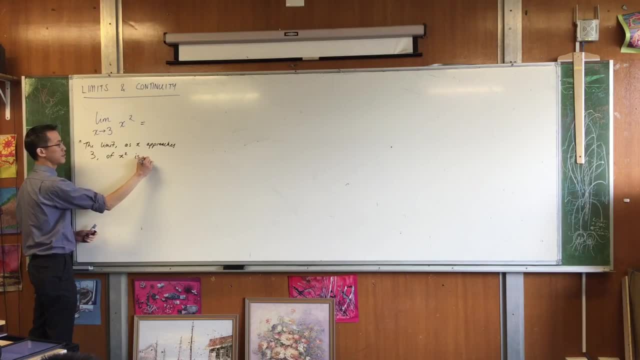 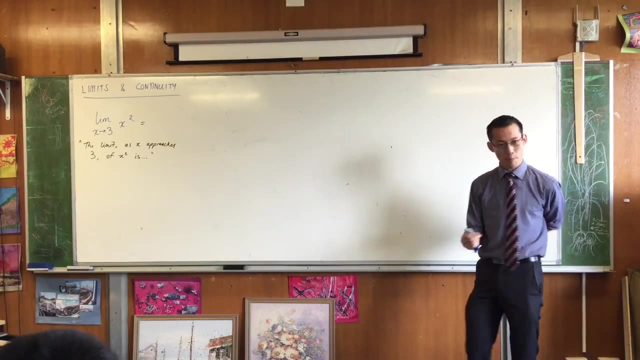 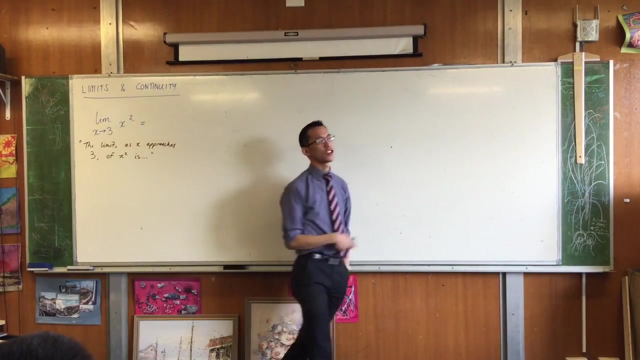 of x squared is. So lim stands for limit. x with an arrow towards 3 says I'm approaching, I'm putting in x values that get closer and closer and closer to 3.. And what I'm putting them into is this particular function up here. 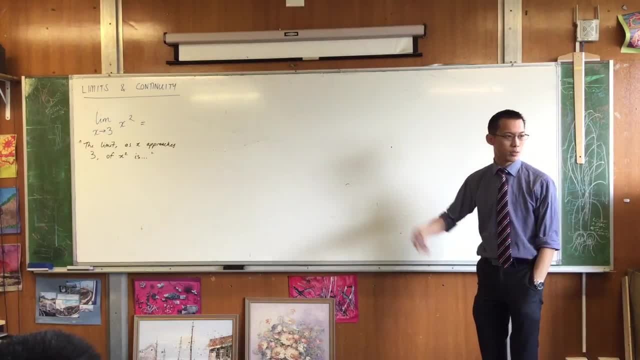 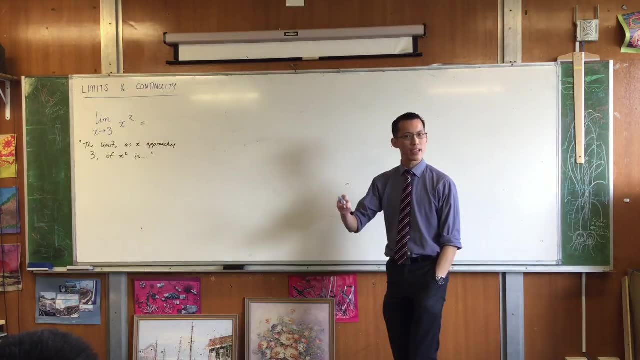 You can have any function you like. I'm just using this as a nice simple example because we can actually work this out. As x gets closer and closer to 3,, what does x squared get closer and closer and closer to Answer? 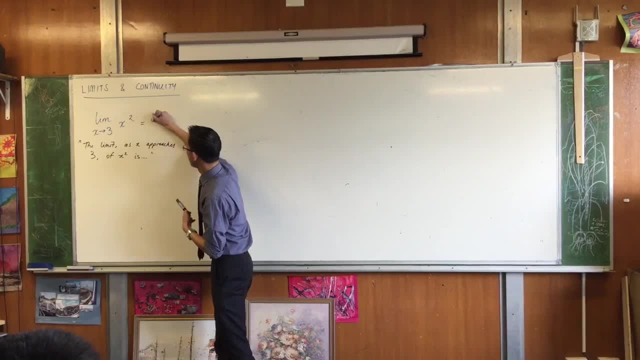 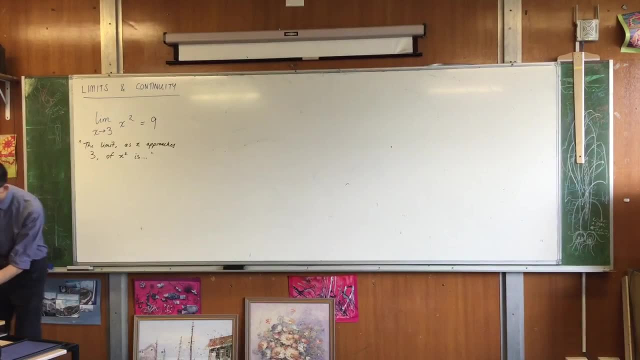 9. So, as the x values change, for example, if I'm going to get my calculator here- if x were 2.9, that's a number that's close to 3.. I don't know what 2.9 squared is, but I'm about to find out. 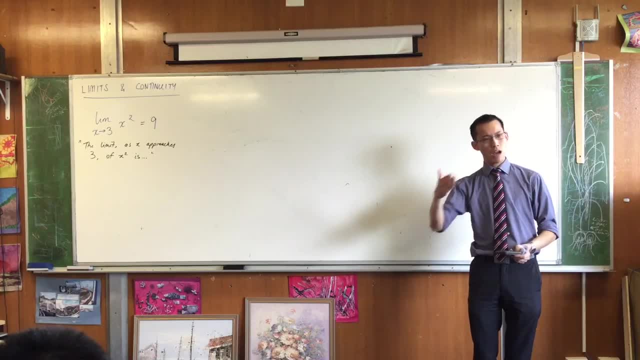 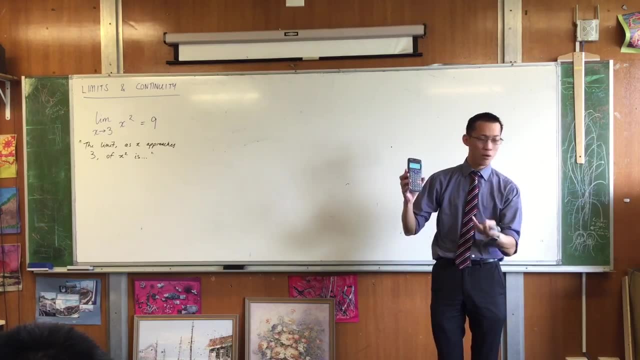 2.9 squared is 8.41. So I'm getting to 9.. If I put in numbers that are closer to 3, like 2.99,, I get 8.9401.. And I can get as close as I like. 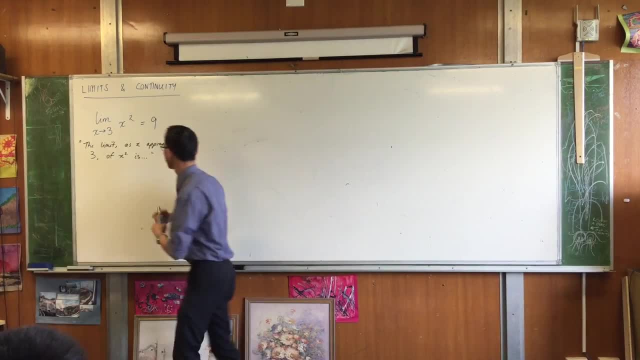 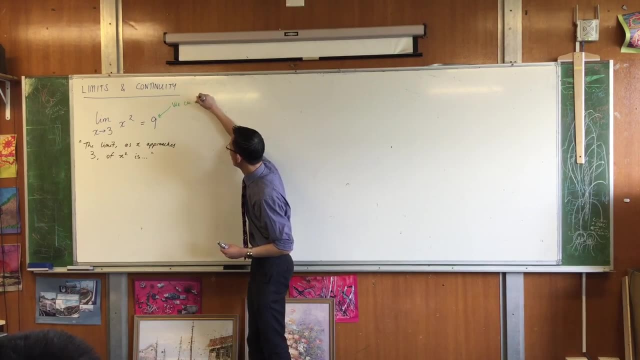 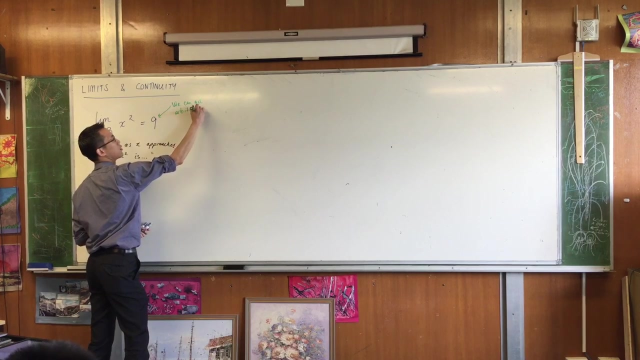 That phrase is actually really important. The reason why 9 is the limit is because we can get the mathematical way of saying it. the technical, rigorous way of saying it is we can get arbitrarily close to this number. So if I say 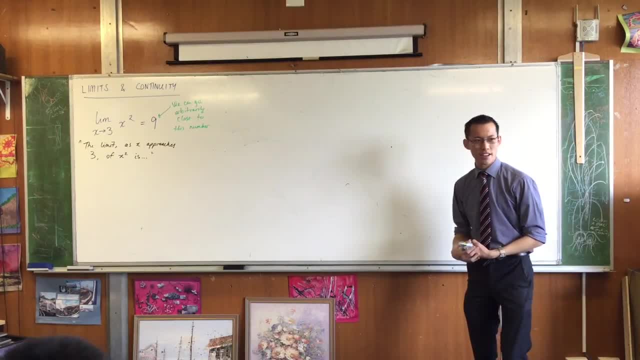 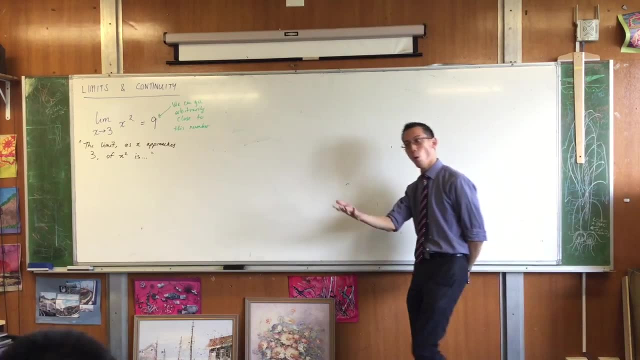 okay, how close would you like to get to 9?? I want to get to 8.9999999999.. That's how close I want to get. You can give me an x value that will get that close or closer right. 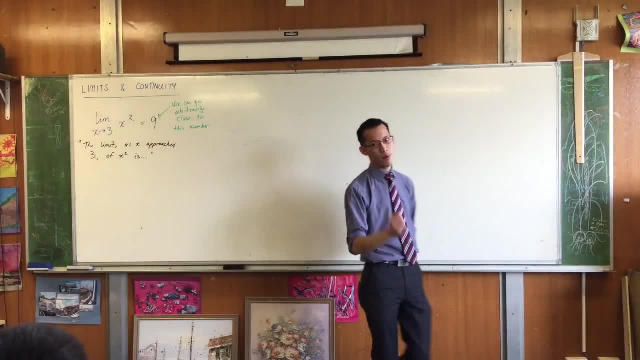 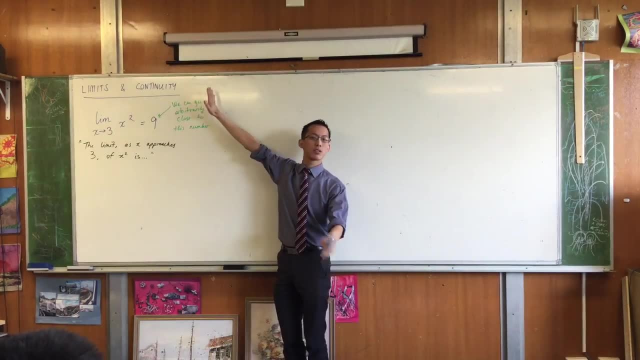 Or 9.0000001.. Is there an x value that can get that close to 9?? And the answer is yes. Yes, there is. I can get arbitrarily close as close as I want. Now, in this case, it's a bit weird. 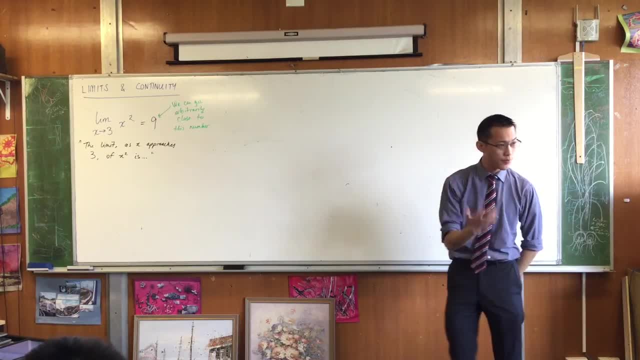 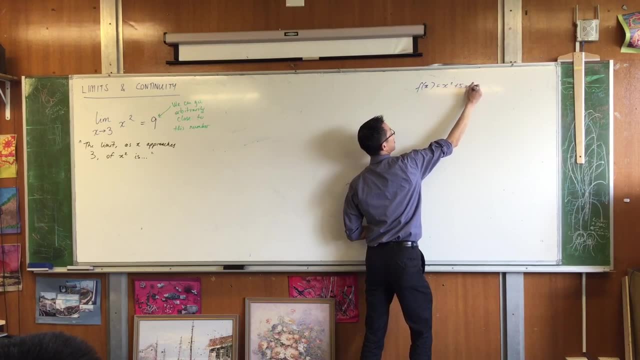 Why do we introduce this notation? I want you to think back to when I introduced function notation. Do you remember? I was like: why are we talking about this when we have perfectly good notation? Why not just say y equals? Why f of x and this weird kind of idea? 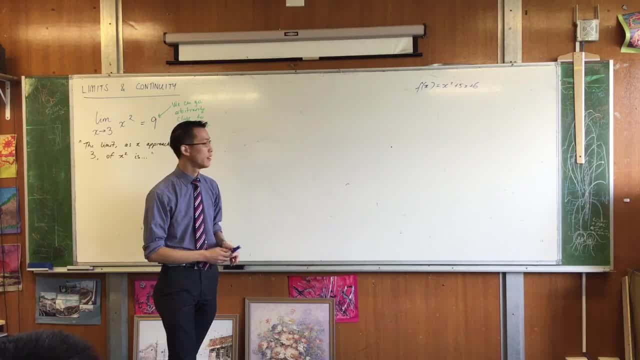 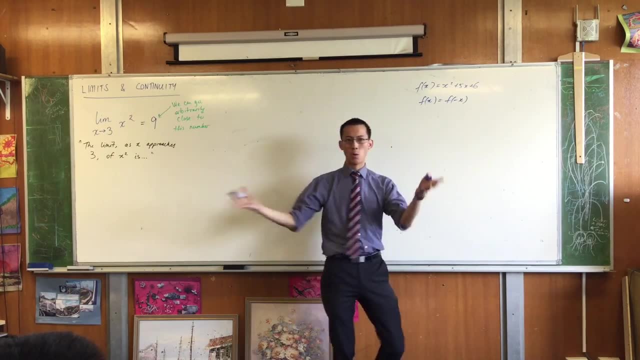 which overlaps with use of brackets and all that kind of thing. that's confusing, And the answer was- at least one of them was: you can talk about things like this. If you have a function where this is true, what do you know about the function? 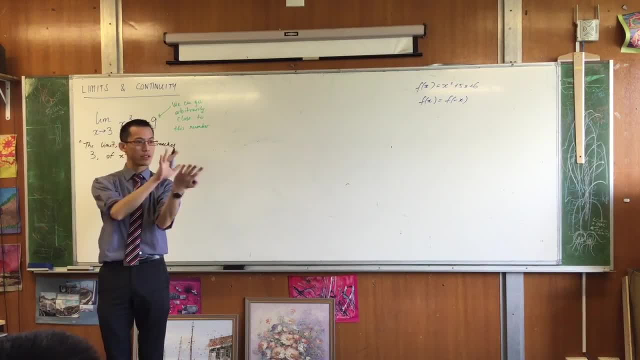 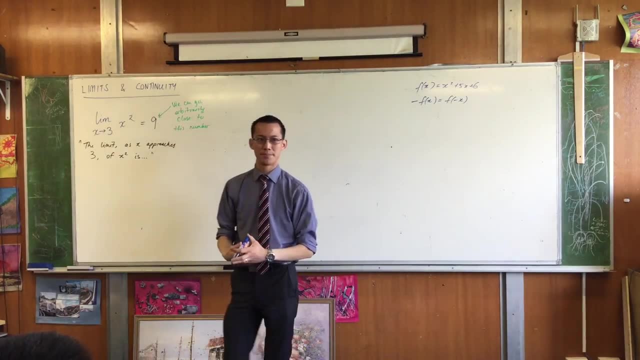 It's an even function. You're going to have line symmetry around the y-axis, right And accordingly, if I say this, what do you know about the function? It's an odd function. It's going to have point symmetry or rotational symmetry. 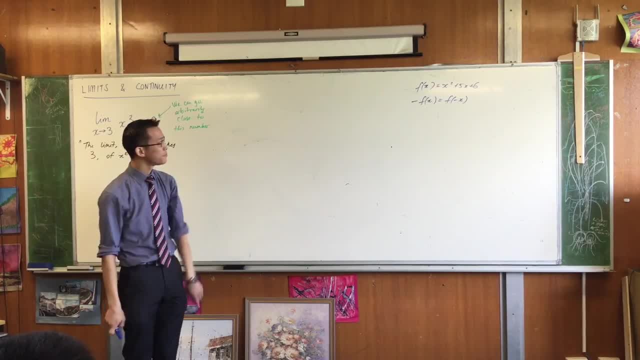 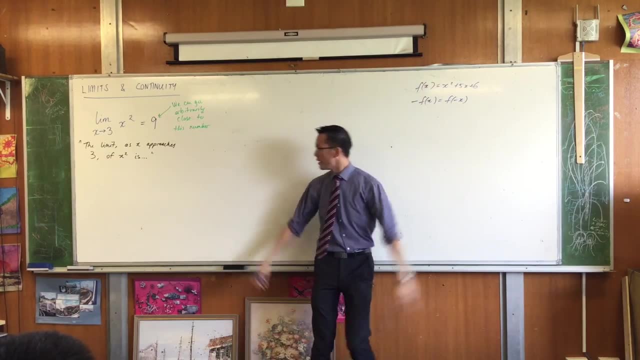 around the origin right, Right at. So when you have that function notation, you can talk about properties that you really couldn't talk about before. It's the same deal with limit notation and limits and continuity, which is a new idea we're going to get into. 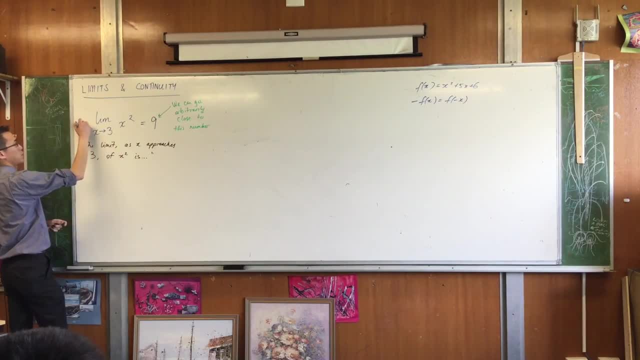 So let me give you some other examples, For instance, this is example one, So example two: Need to introduce a bit more notation here. So if I say limit as x approaches infinity- we've talked about this before in the context of graphing right- 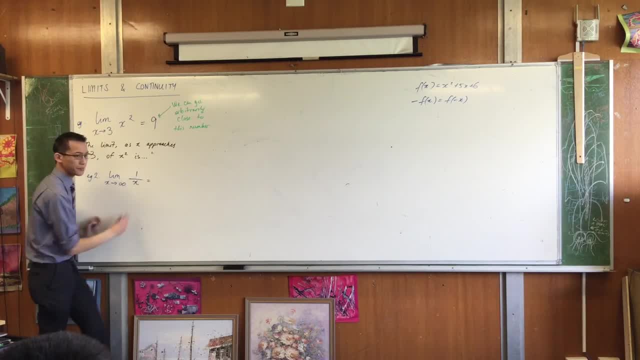 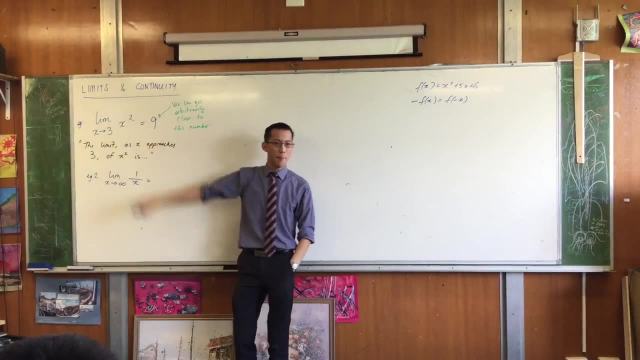 So I might say something like this: Okay Now, this is important as an example, because, unlike this one right, Unlike this example where you could have gotten nine just by putting in x equals three, You can actually substitute it in. You cannot substitute in x equals infinity. 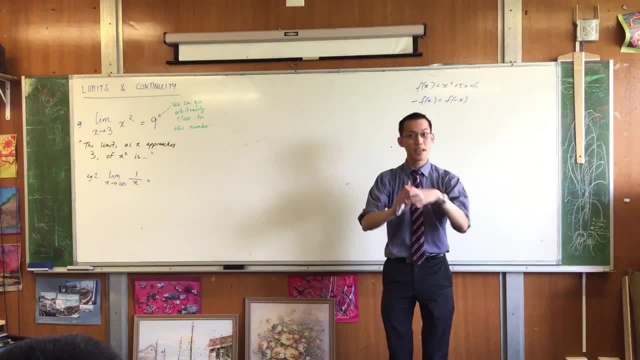 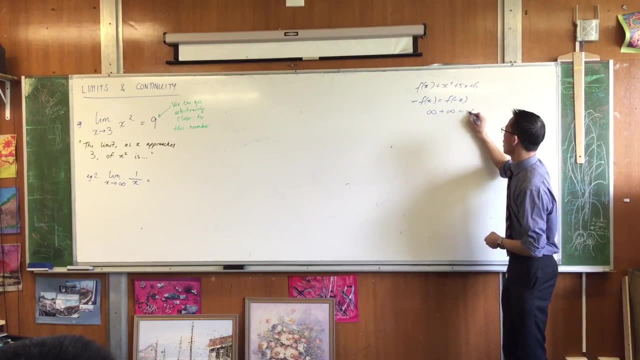 because infinity is not a number, It's a concept, It's an idea. It behaves a little bit like a number, but in other ways it does not right. So you're like: what do I do with this thing? The arithmetic of infinities is a tricky thing. 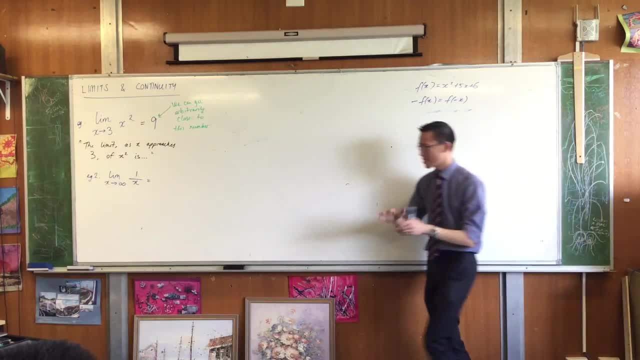 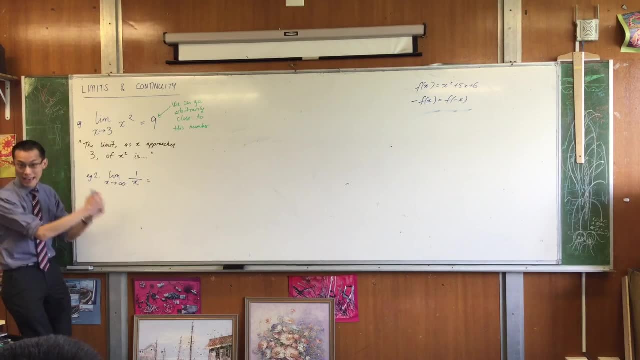 that is not within the scope of this course, but we can still understand the idea. as x gets enormous, This becomes one over an enormous number. What's one over an enormous number Now? I want you to notice how this fits into this. 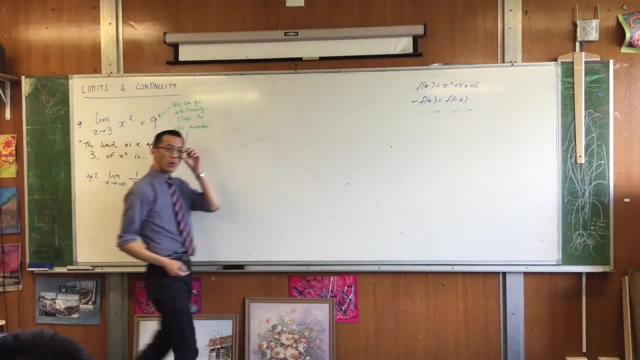 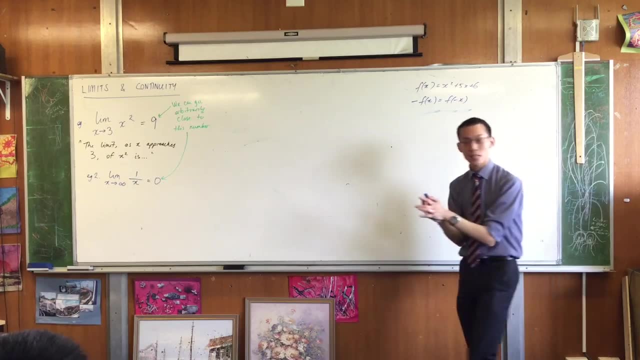 Okay, The function one over x. If I want to get to a value like 0.00000000001,. is there an x value that can get to that? The answer is yes, No matter how close you get to 0,. 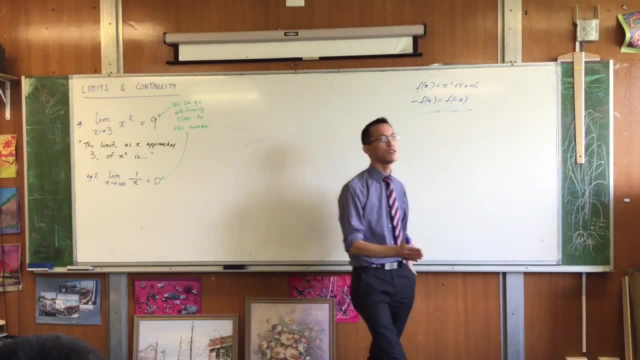 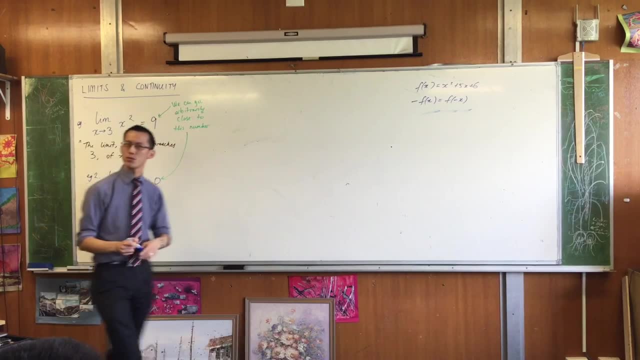 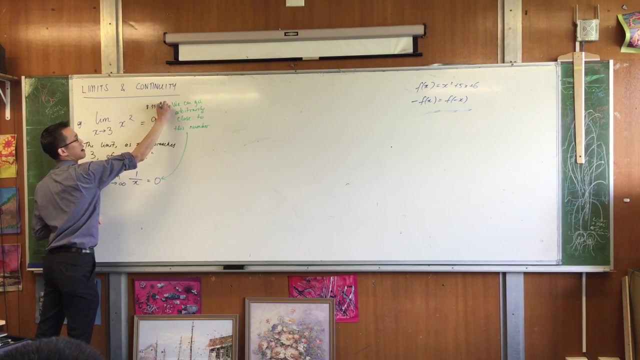 arbitrarily close. you can find an x value that'll do that- Okay. But when you start thinking about this function here immediately you come into some problems. So one of the important things about this is you remember I said you can approach and get really, really small. 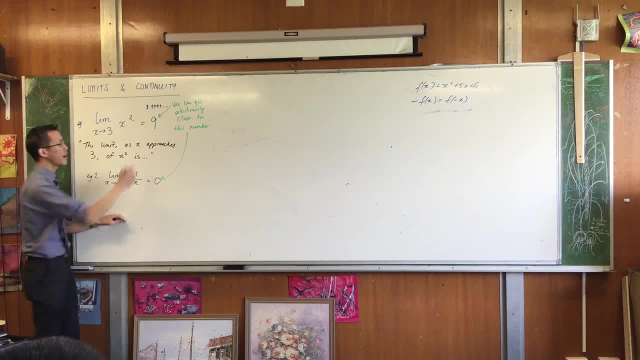 sorry, really, really close values below nine and you can also get really close values above Right. So when you come from one direction, I used to be able to say that name with a straight face. Anyway, when I come from one direction, 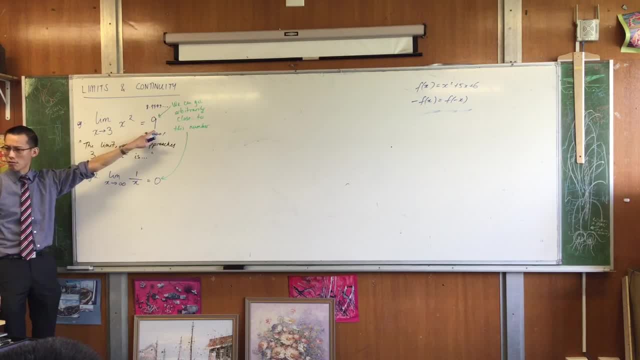 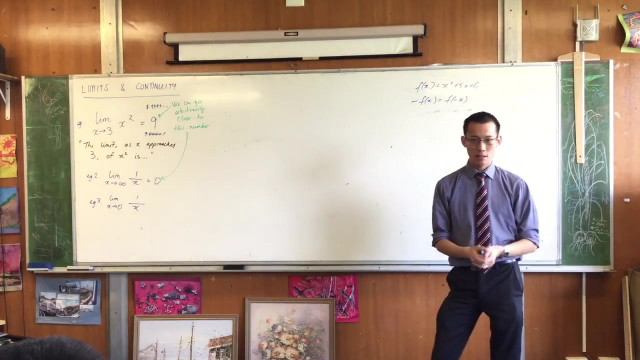 or I come from the other direction. you come to the same value. But when you think about this guy- this is an important case study for us- you run into a problem. You know what this graph looks like. You know what it looks like, right. 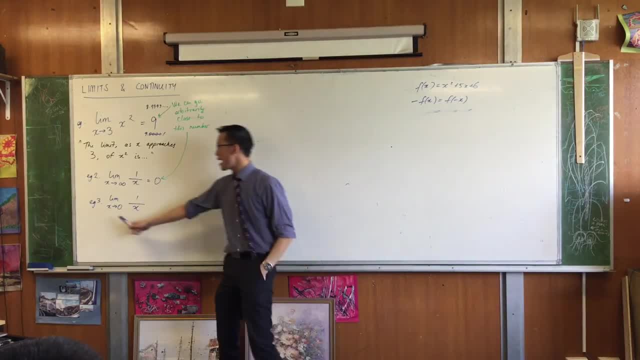 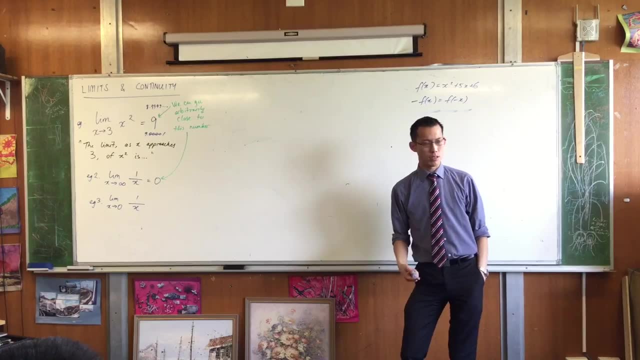 It's got two branches right. So when you say, hey, when x gets closer and closer to 0, what does this thing approach? You sort of run into this snag. How do you state the answer? Let's just underneath draw the graph. 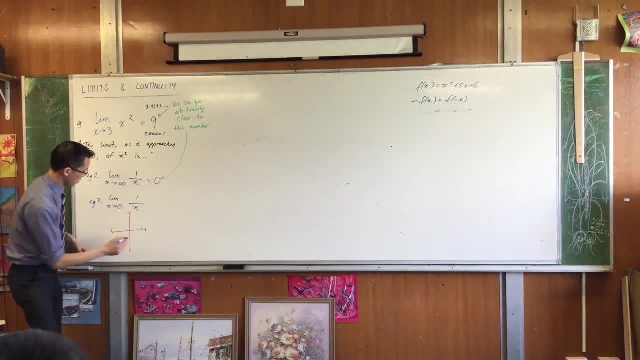 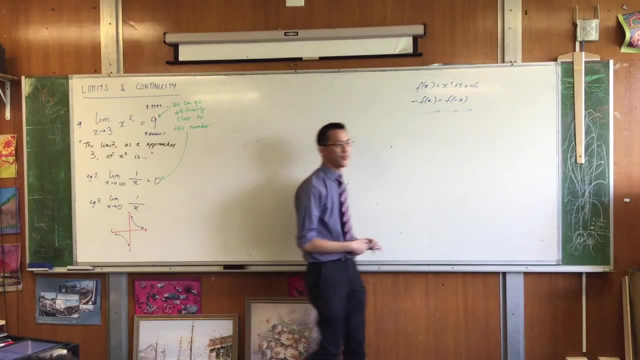 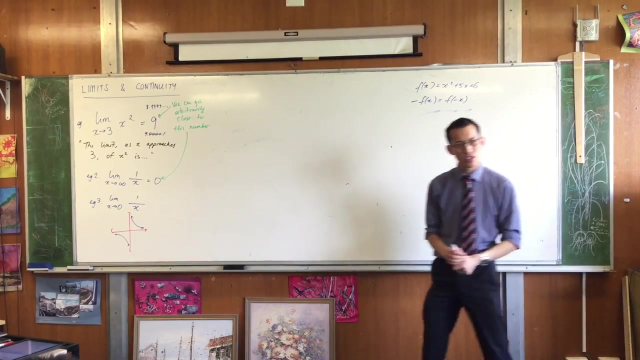 in a small version, is all enough. Now, when x is approaching positive infinity, the limit which is unambiguously 0, there's nothing else that it approaches, okay. But when you get closer to 0, well, if you try putting in positive values, 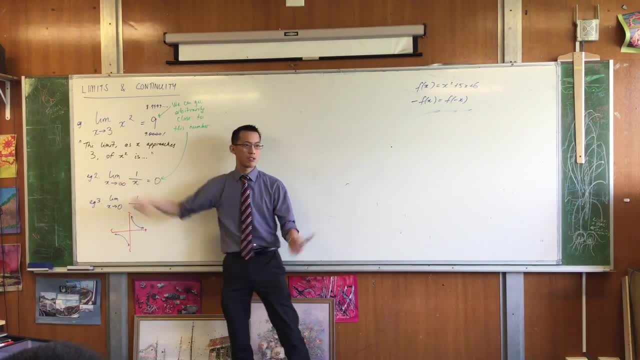 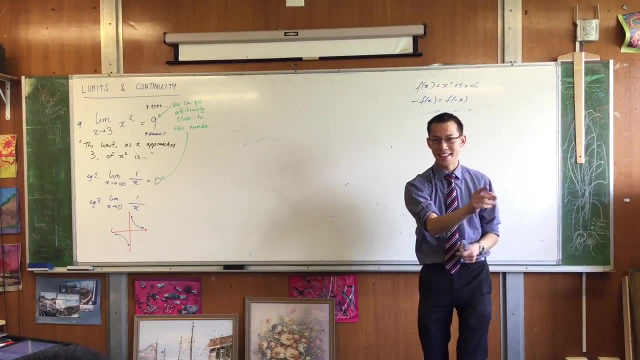 that are close to 0,, like 0.1 or 0.01,, et cetera. what are you going to approach? You're going to approach a huge number, In fact. now, this is weird. This is where it's similar but different. 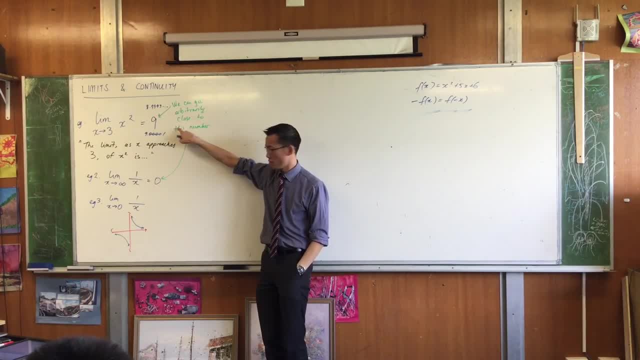 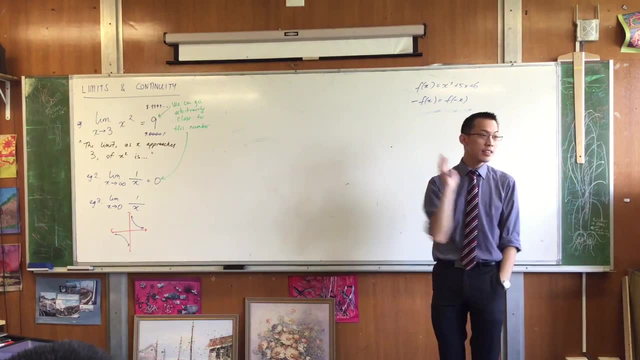 You can become arbitrarily close to positive infinity right, Give me a number, a million, a billion, a Google, anything you like. I can give you an x value that will get to that. 1 over x will get up to there, okay. 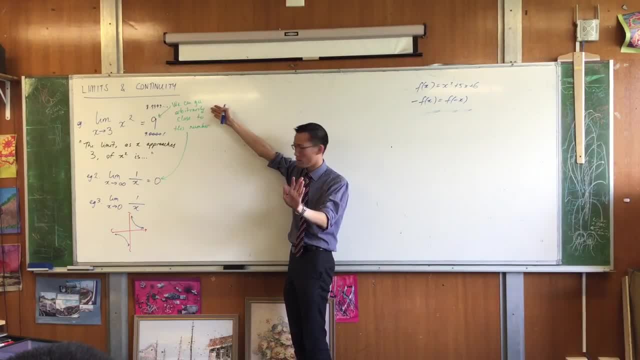 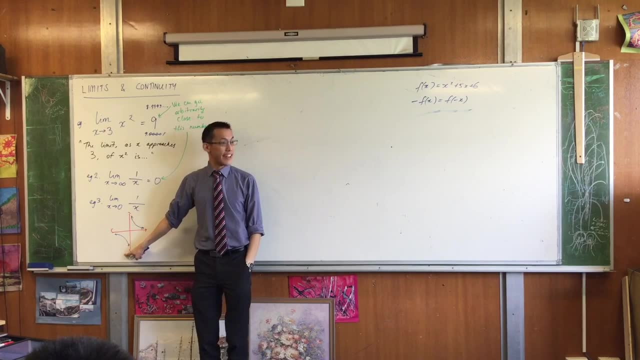 So I can get arbitrarily close, I can get as big as you like. okay, That's what happens when you put in 0.0001 or whatever. But when you put in negative 0.0001 or those kinds of things. 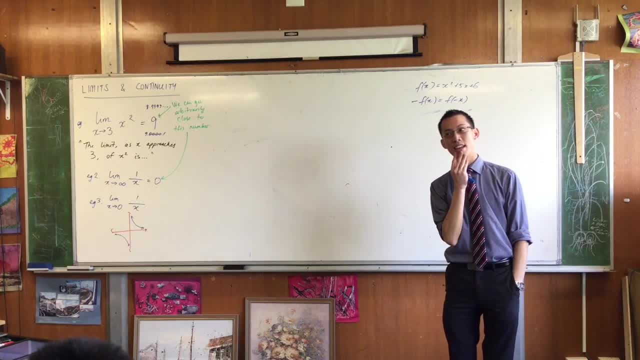 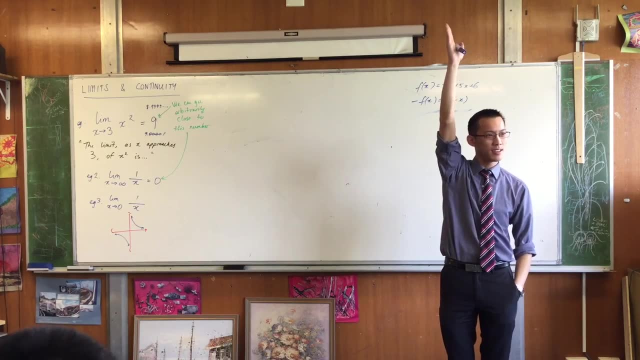 you do not approach negative infinity, do you? You instead approach? Sorry, did I say that right? Yeah, I said the answer because I was thinking the answer: You don't approach positive infinity, You approach negative infinity because it's dropping like a rock down here. okay, 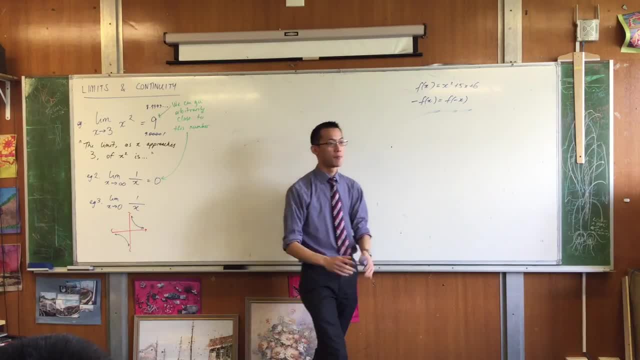 So therefore, this, as it's stated, has no answer. There is no limit. Mean girls is that where that comes from? The limit doesn't exist, okay, However, this concept is still important to us, so we distinguish between: 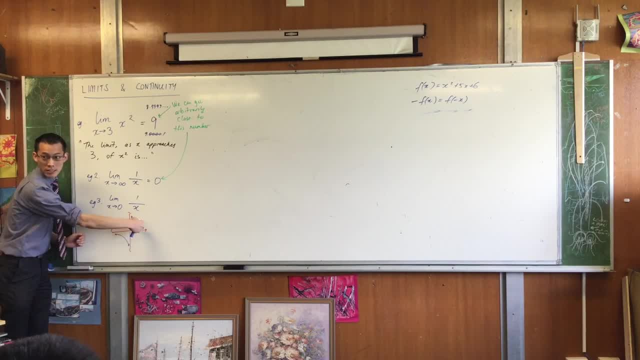 approaching 0 from the positive side, like this, or approaching 0 from the negative side. Here's some new notation for you: When you put a plus sign in the index right In the power, as if it were a power. 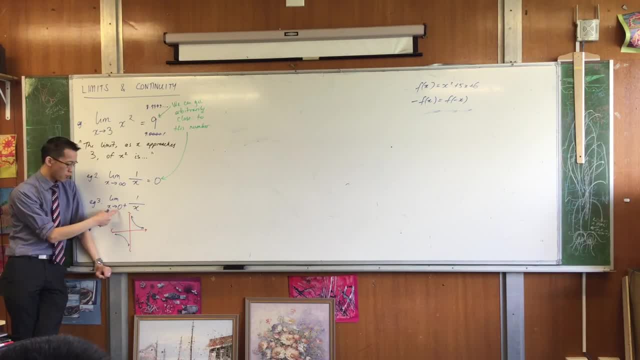 It's not a power, because it's not even a number. okay, What this means is you're approaching 0 from the positive side, That's from right to left, Does that make sense? So this is approaching from the right, so therefore, this is equal to positive infinity, okay.